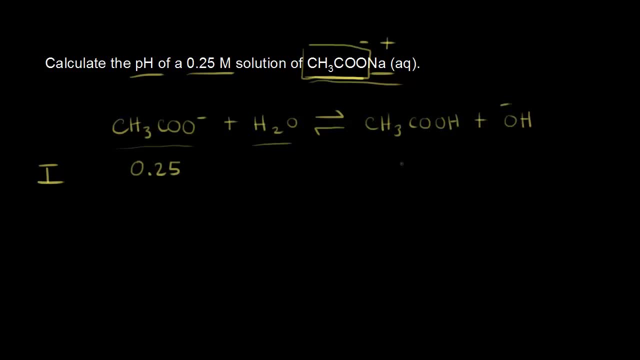 And if we pretend like nothing has reacted, we should have a zero concentration for both of our products. So a zero concentration for our two products. Next, we're going to calculate the pH of our solution. First we think about the change. 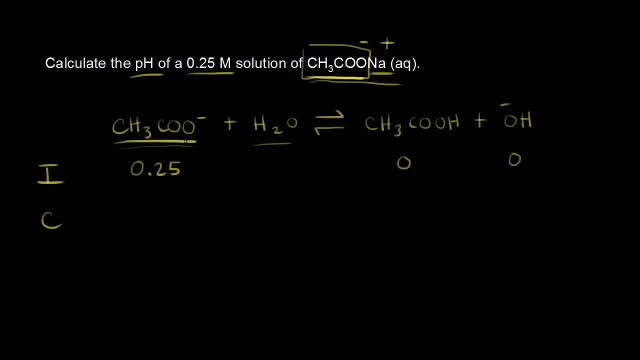 So CH3COO-, the acetate anion, when it reacts is going to turn into CH3COOH or acetic acid. So whatever concentration we lose for the acetate anion, we gain for acetic acid. So if we make the concentration of the acetate anion X that reacts, 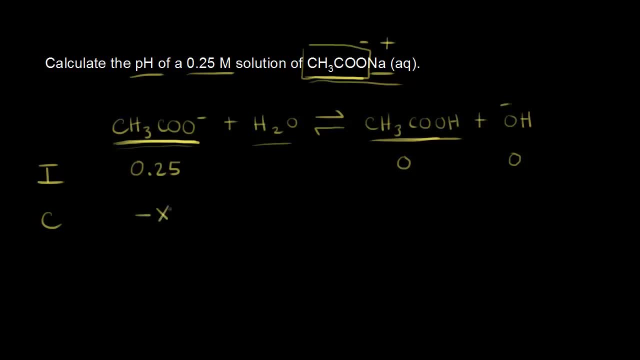 so if X reacts, if X concentration reacts, we're going to lose X And we're going to gain X over here. And it's the same thing for hydroxide: We would be gaining X, a concentration for the hydroxide. 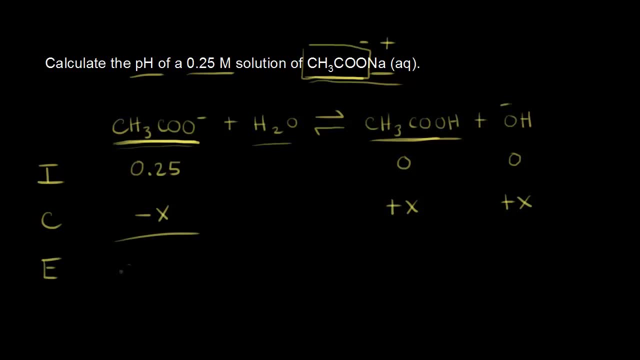 So at equilibrium the concentration of acetate would be 0.25 minus X. So we're assuming everything comes to equilibrium here. The concentration of acetic acid would be X. The concentration of hydroxide would also be X. Next we write our equilibrium expression: 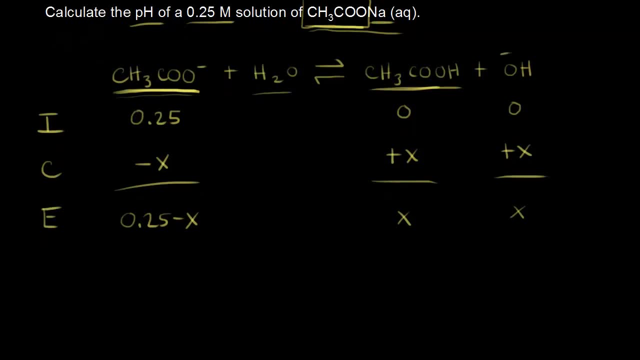 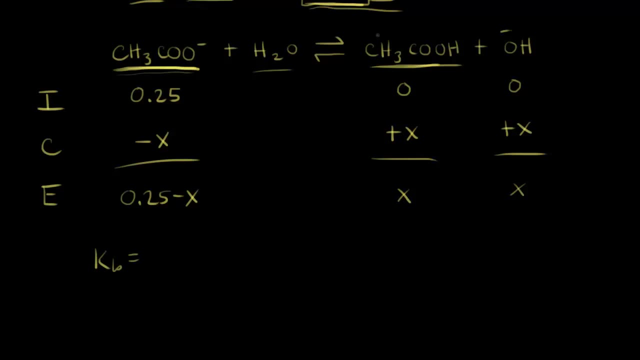 And since this is acetate functioning as a base, we write KB here. So we write KB is equal to concentration of our products over concentration of our reactants. So we have the concentration of CH3COOH times the concentration of hydroxide. 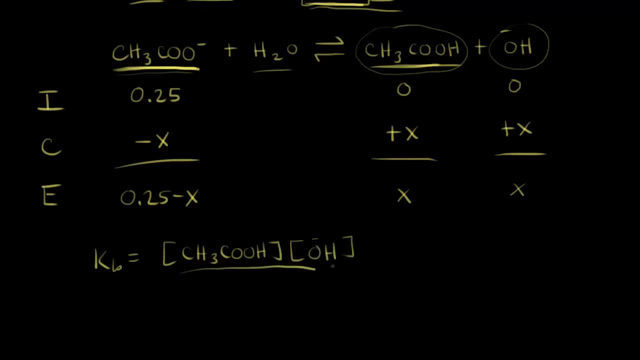 so times the concentration of OH- this is all over the concentration of our reactants. And once again we ignore water. So we have only the concentration of acetate to worry about here. So we put in the concentration of acetate, Alright. so let's think about the concentration of acetic acid at equilibrium. 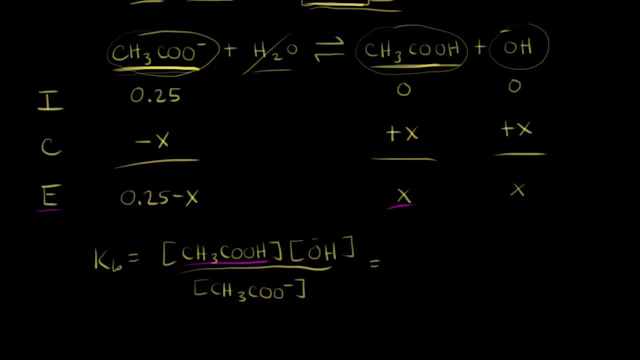 So at equilibrium the concentration is X, So I go over here and put X And then for hydroxide it's the same thing. The concentration of hydroxide at equilibrium is also X, So I put X in over here. 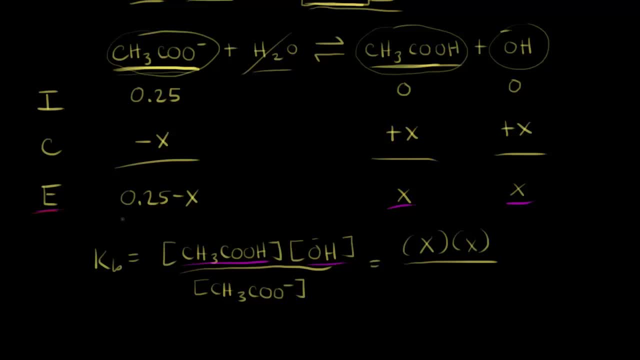 And then for the concentration of acetate. at equilibrium, the concentration of acetate is 0.25 minus X- 0.25 minus X. Next, we need to think about the KB value for this reaction, And you will probably not be able to find this in any table. 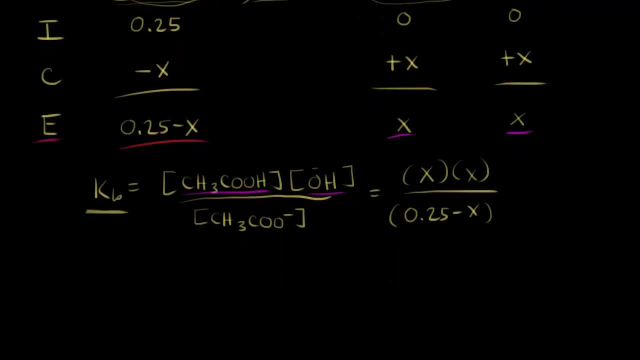 but you can find the Ka for acetic acid, So acetic acid, right acetic acid and acetate. this is a conjugate acid base pair And the Ka value for acetic acid is easily found in most textbooks And the Ka value is equal to 1.8 times 10 to the negative 5.. 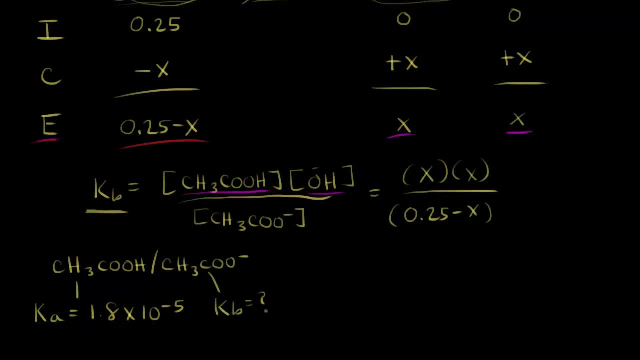 And our goal is to find the KB right. what is the KB for the conjugate base? And we know that for a conjugate acid base pair, Ka times KB is equal to Kw, right the ionization constant for water. So we can go ahead and plug in 1.8 times 10 to the negative 5. 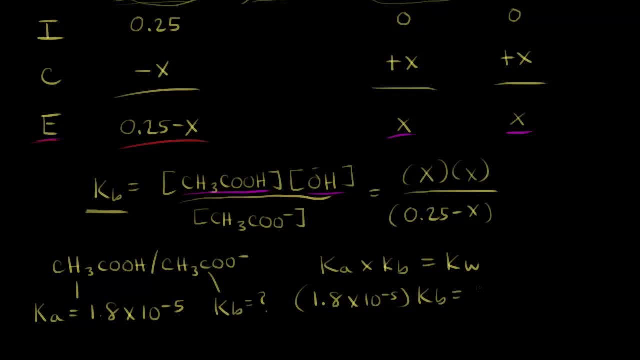 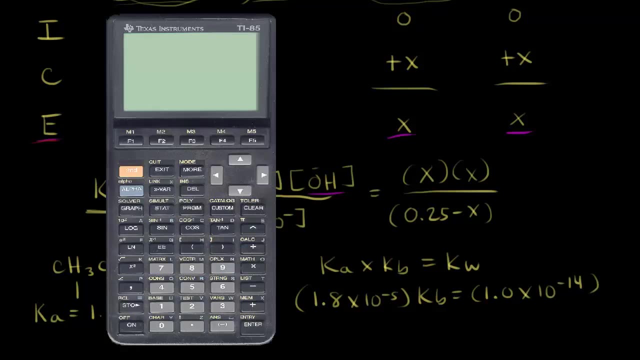 times KB. It's equal to. we know this value is 1.0 times 10 to the negative 14.. So we just need to solve for KB So we can get out the calculator here and take 1.0 times 10 to the negative 14.. 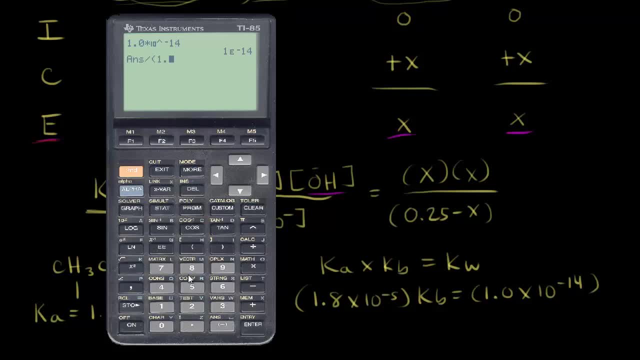 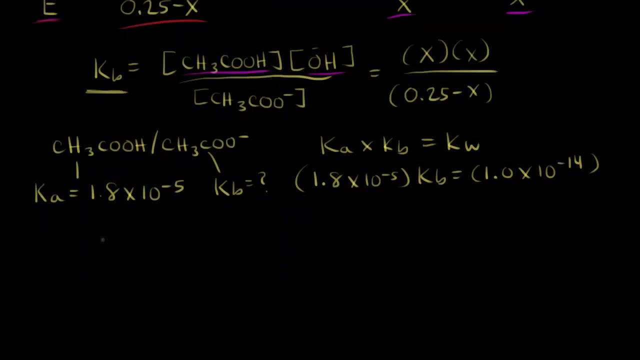 And then we divide by 1.8 times 10 to the negative 5. And so we get 5.6 times 10 to the negative 10.. So let's get some more space down here and let's write that. So KB is equal to 5.6 times 10 to the negative 10.. 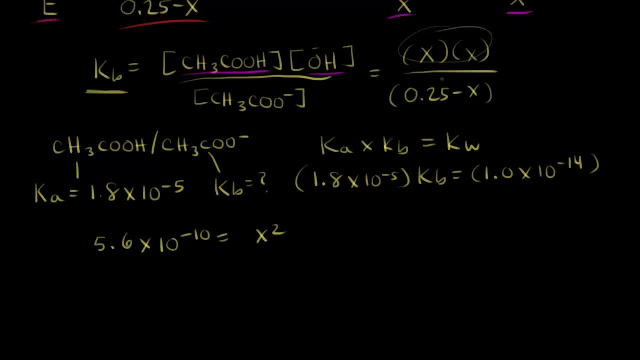 And this is equal to x squared right is equal to x squared over 0.25 minus x. Next, to make the math easier, we're going to assume that the concentration x is much, much smaller than 0.25.. 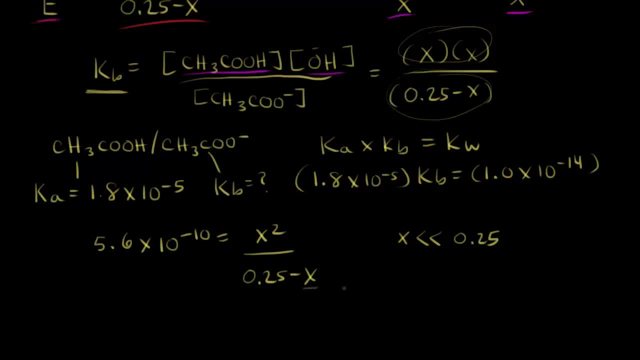 And if that's the case, right, if this is an extremely small number, we can just pretend like it's pretty close to 0. And so 0.25 minus x is pretty much the same thing as 0.25.. So let's make that assumption once again. 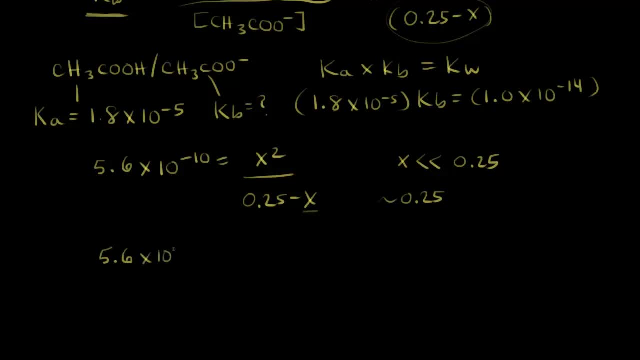 to make our life easier. So this is 5.6 times 10 to the negative 10.. It's equal to x squared over 0.25.. So now we need to solve for x. All right, so we have 5.6 times. 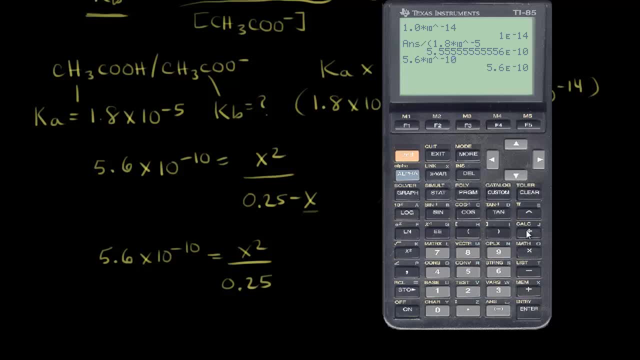 10 to the negative 10.. And we're going to multiply that. we're going to multiply that by 0.25.. And so we get 1.4 times 10 to the negative 10.. So we now need to take the square root of that number. 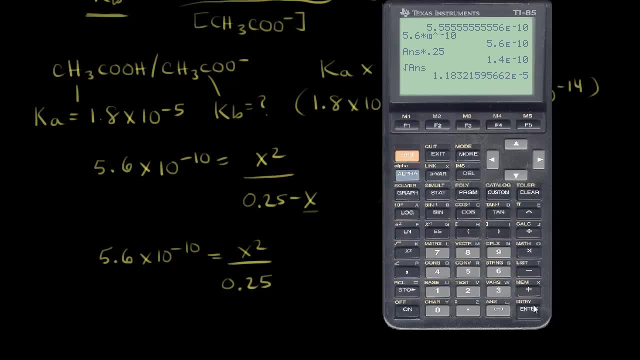 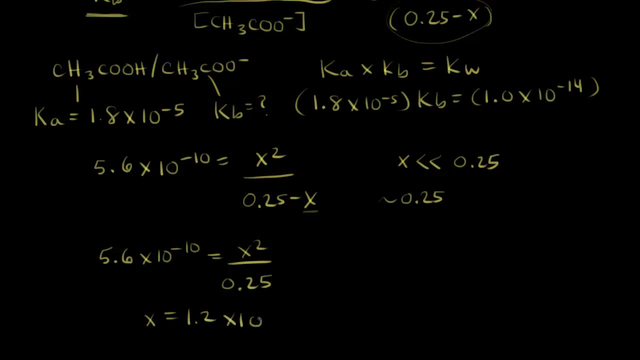 all right, and we get x is equal to. this gives us: x is equal to 1.2 times 10 to the negative 5.. So let's go ahead and write that here. So x, x is equal to 1.2 times 10 to the negative 5.. 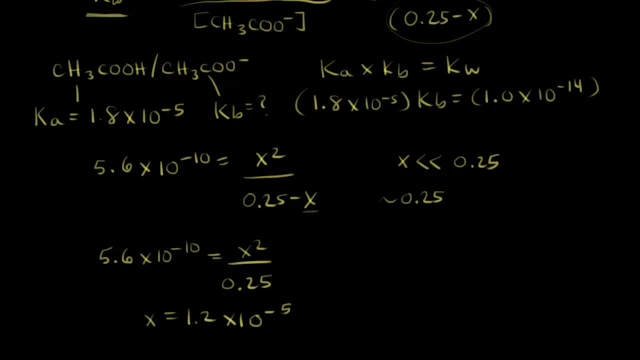 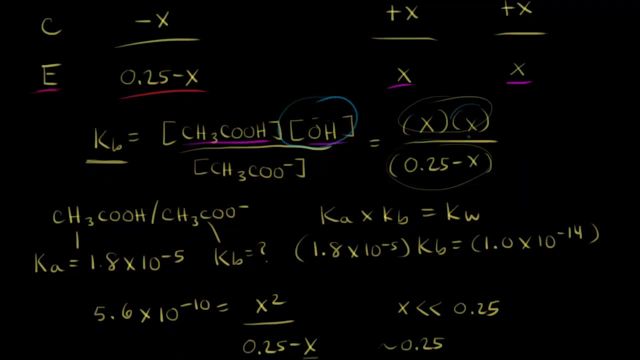 All right, what did x represent? We have all these calculations written here. We might have forgotten what x represents. x represents the concentration of hydroxide ions, right? So x is equal to the concentration of hydroxide ions, So let's go ahead and write that down. 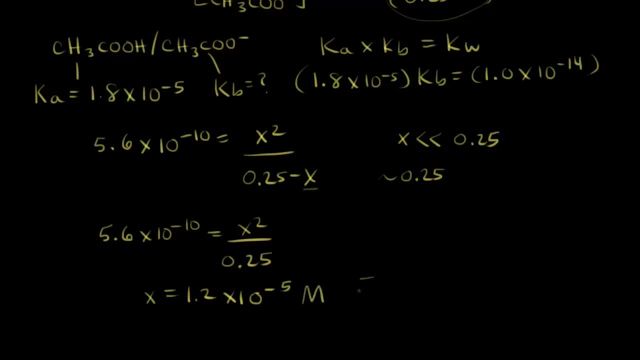 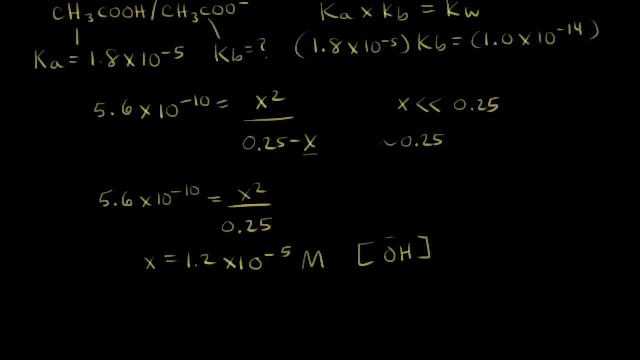 x is equal to the. so this is molarity, this is the concentration of hydroxide ions, And if we know that, we can eventually get to the pH right. That was our original question: calculate the pH of our solution. 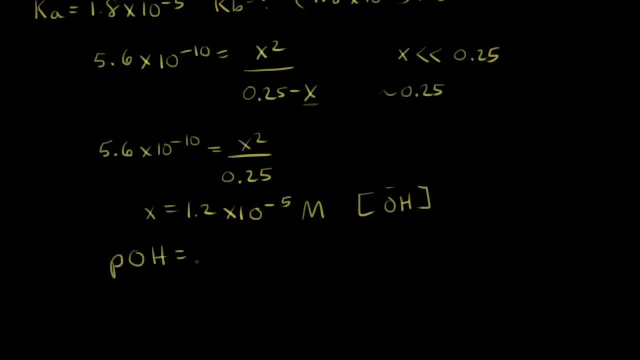 So we could find the pOH from here. I know the pOH is equal to the negative log of the hydroxide ion concentration, So I can take the negative log of what we just got. so the negative log of 1.2 times 10 to the negative 5,. 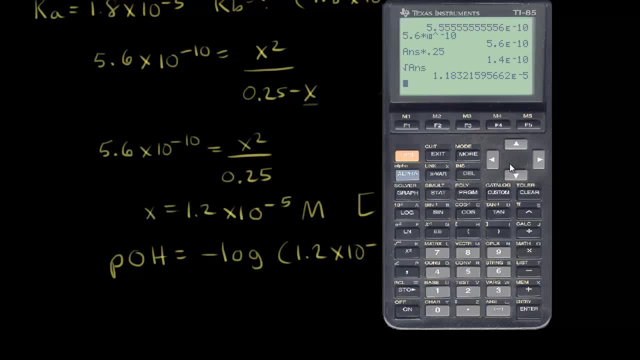 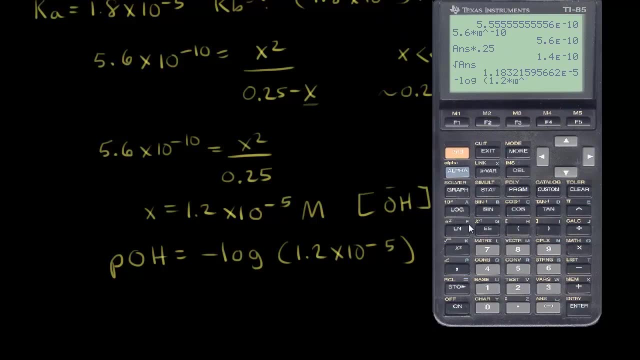 and that will give me the pOH. All right, so let's go ahead and do that. So the negative log of 1.2 times 10 to the negative 5 is going to give me a pOH of 4.92.. 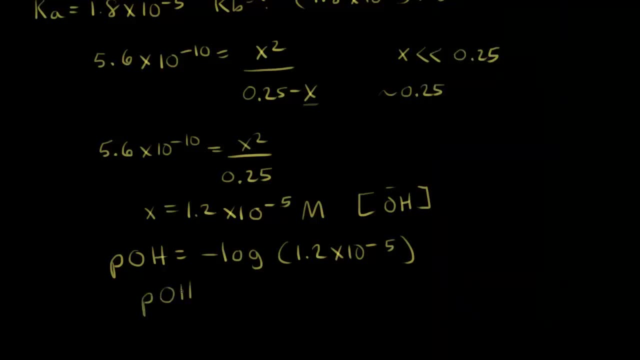 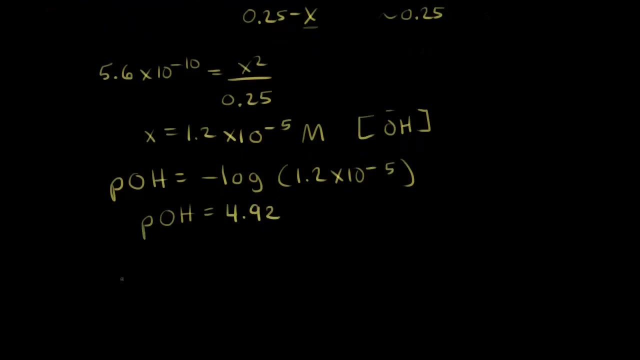 All right, so I go ahead and write: pOH is equal to 4.92.. And finally, to find the pH, I need to use one more thing, because the pH plus the pOH is equal to 14.. All right, so I can plug in the pOH into here. 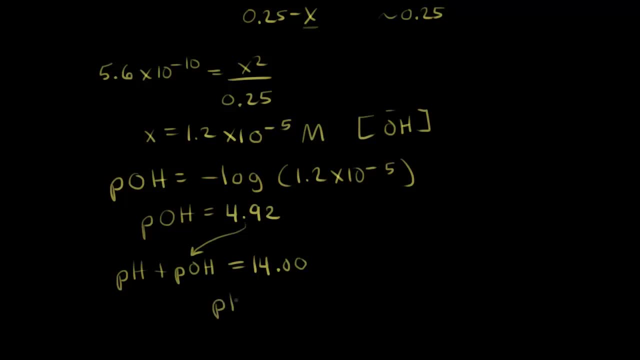 and then subtract that from 14, so the pH is equal to 14 minus 4.92, and that comes out to 9.08.. So the pH is equal to 9.08.. So we're dealing with a basic solution for our salt. 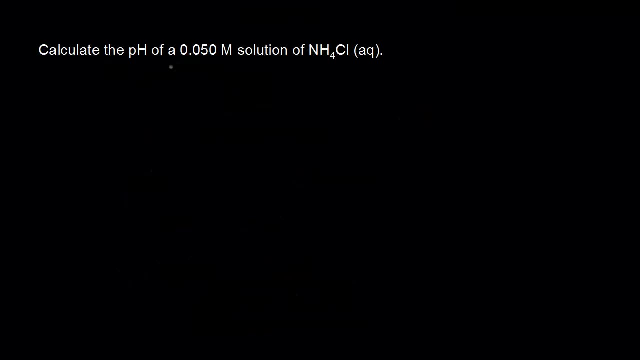 Let's do another one. So our goal is to calculate the pH of a .050 molar solution of ammonium chloride. So for ammonium chloride we have NH4 plus and Cl minus. The chloride anions aren't going to react appreciably with water. 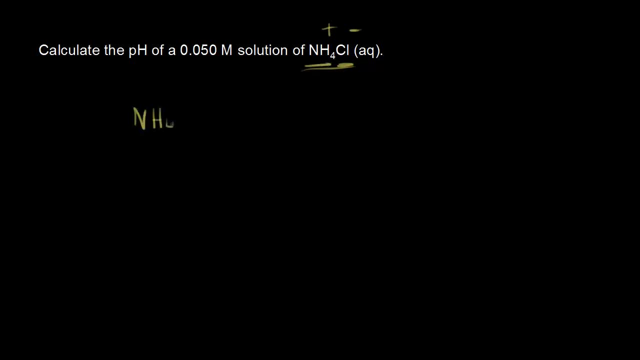 but the ammonium ions will. So let's write our reaction here. So NH4 plus is going to function as an acid. It's going to donate a proton to H2O. So if H2O accepts a proton, that turns into hydronium ions. 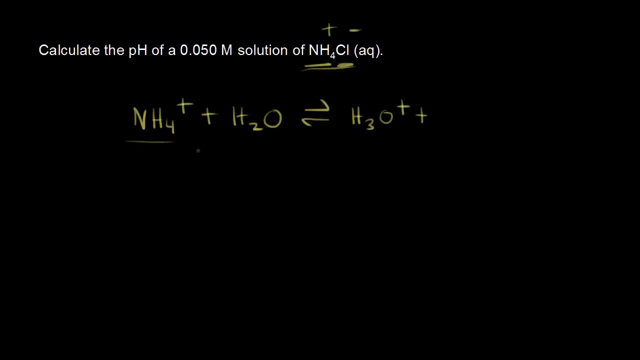 so H3O plus, And if NH4 plus loses a proton, we're left with NH3.. All right, so let's start with our initial concentrations. Well, we're trying to find the pH of our solution and we're starting with .050 molar solution. 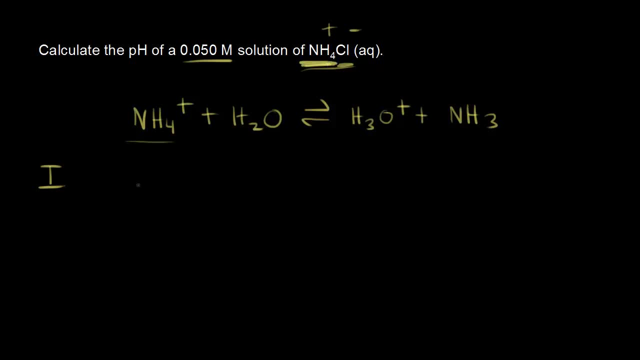 of ammonium chloride. So that's the same concentration of ammonium ions, right? So this is .050 molar, And if we pretend like this reaction hasn't happened yet, our concentration of our products is zero. Next we think about the change. 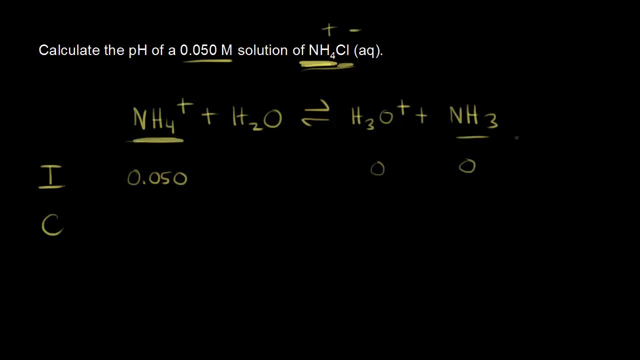 And since NH4 plus turns into NH3, whatever we lose for NH4 plus is what we gain for NH3.. So if we lose a certain concentration of X for ammonium, right, if we lose a certain concentration of X for NH4 plus. 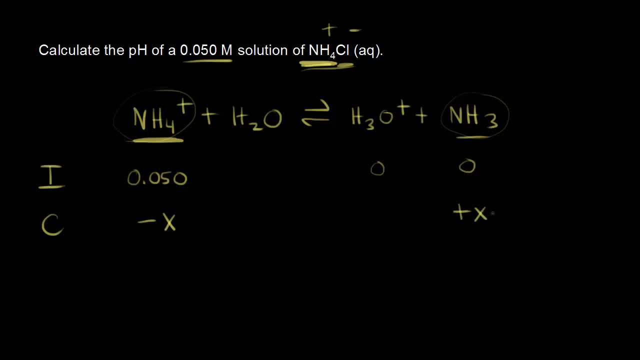 we gain the same concentration- X- for NH3. And therefore we'd also gain the same concentration for hydronium as well. So at equilibrium our concentration of ammonium would be .050 minus X For the hydronium ion. 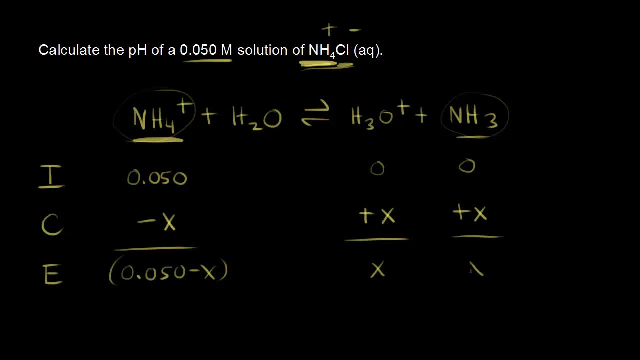 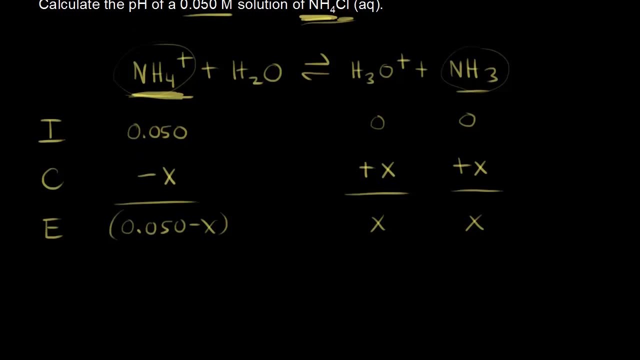 it would be X. And for ammonia, for NH3, it would be X as well. So we're talking about ammonium acting as an acid here, And so we're going to write an equilibrium expression. We're going to write Ka. 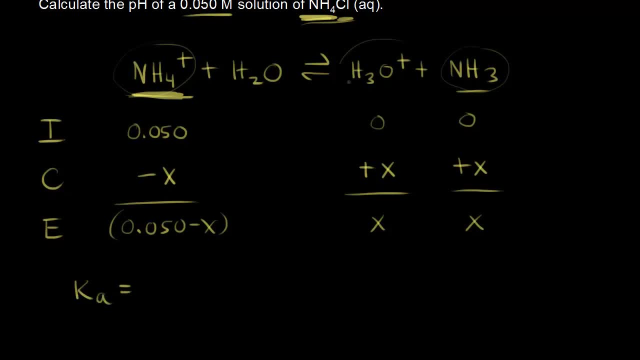 So Ka is equal to concentration of products over reactants. So this would be the concentration of H3O plus times the concentration of NH3, all over the concentration of NH4 plus, because we're leaving water out, So all over the concentration of NH4 plus. 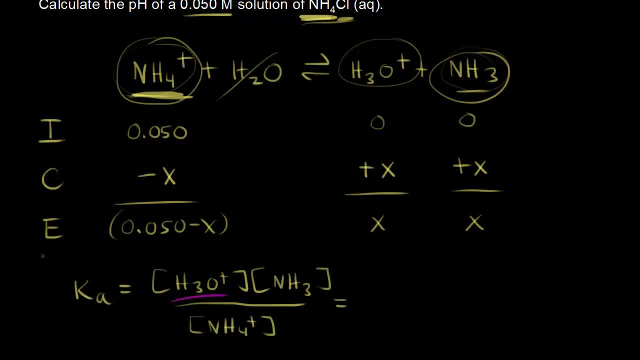 All right. The concentration of hydronium ions at equilibrium is X, So we put an X in here. Same thing for the concentration of NH3, right, That would be X, So we put an X into here. This is all over the concentration. 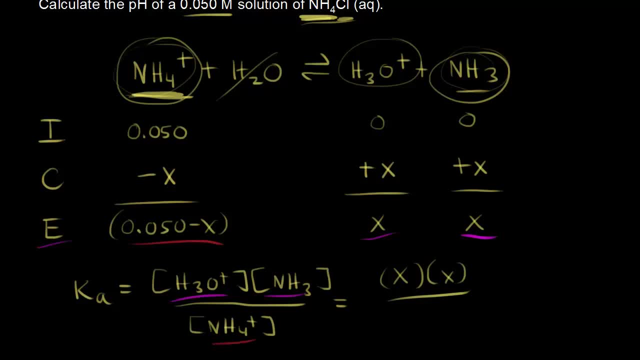 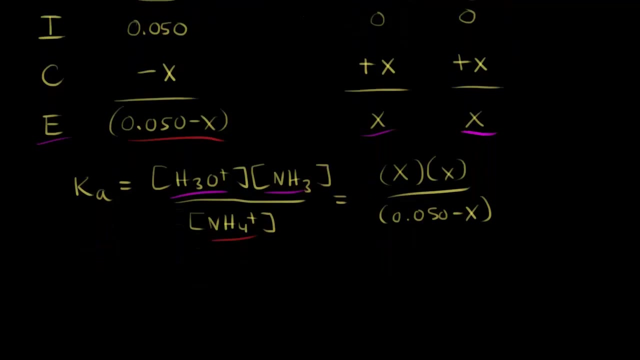 of ammonium, which is .050 minus X. So over here we put 0.050 minus X. Now next we need to think about the Ka value. All right, So finding the Ka for this reaction is usually not something you would find. 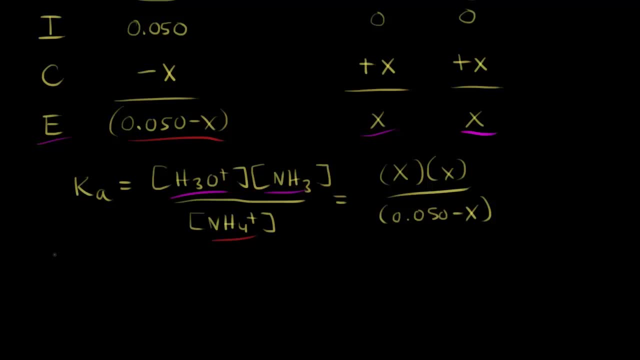 in a table, in a textbook. But we know that we're talking about an acid base, a conjugate acid base pair, here. So NH4 plus and NH3 are a conjugate acid base pair. We're trying to find the Ka for NH4 plus. 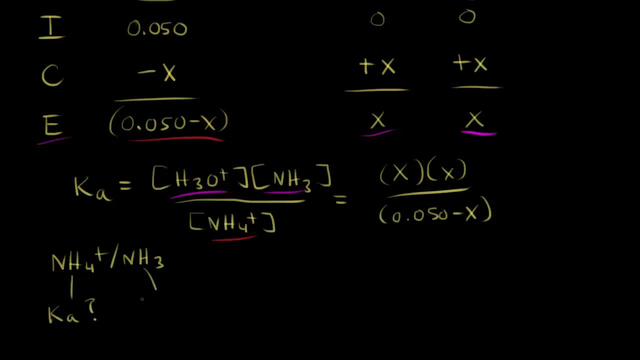 And again, that's not usually found in most textbooks. But the Kb value for NH3 is it's 1.8 times 10 to the negative five. So for a conjugate acid base pair, Ka times Kb is equal to Kw. 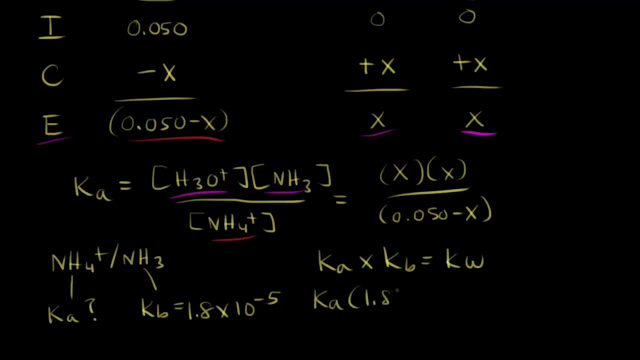 So we're trying to find Ka. We know Kb is 1.8 times 10 to the negative five. This is equal to 1.0 times 10 to the negative 14.. So we can once again find find Ka on our calculator. 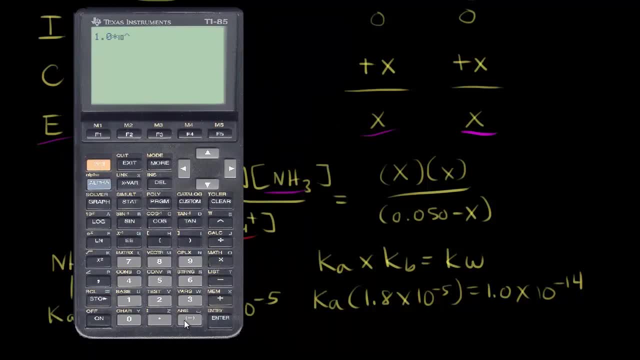 So 1.0 times 10 to the negative 14.. We divide that by 1.8 times 10 to the negative five, And so the Ka value is 5.6 times 10 to the negative 10.. So if we get some room down here, 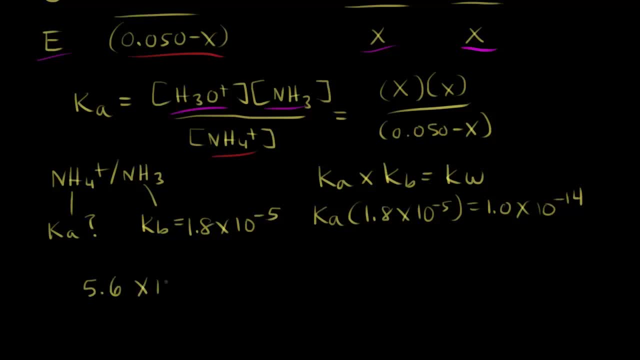 we say Ka is 5.6 times 10 to the negative 10.. This is equal to. this would be x squared over here And once again, we're going to assume. we're going to assume that x is much, much smaller than 0.050.. 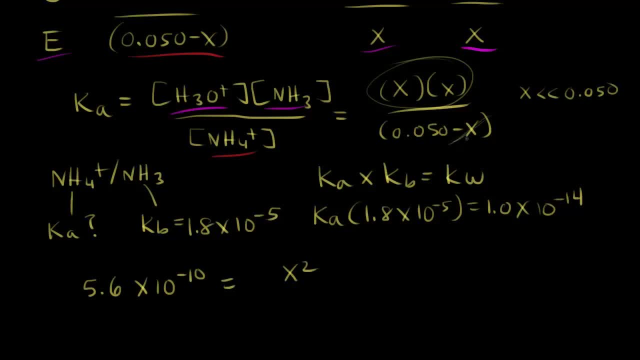 So we don't have to worry about x right here. If it's an extremely small number, 0.050 minus x is pretty much the same as 0.050.. So we plug this in and we have 0.050 here.